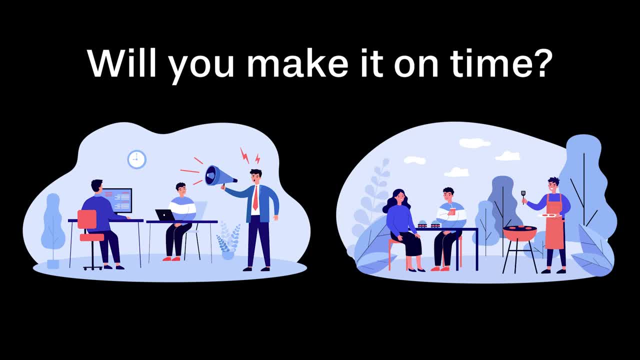 So, in pondering what to do next, you ask yourself what is the chance that you could even finish these two reports in time for the party, and how could you actually even go about computing that chance? Now, to answer this question, we are going to rely on Monte Carlo, Simulation And what's. 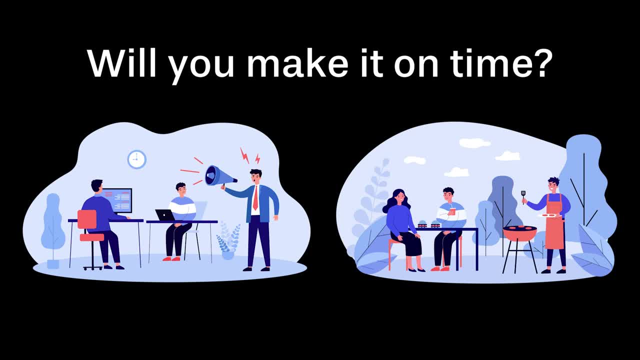 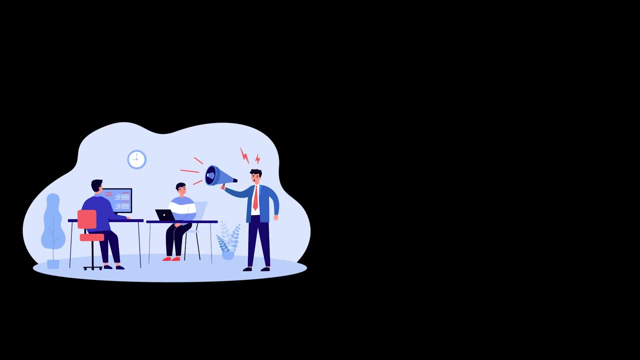 wonderful about this technique is that we can answer challenging probabilistic questions like this one with limited background, actually in probability. So let's go back to our situation. Todd is expecting that you have two reports on his desk by end of day. Based on past experience, you're going to make a couple of guesses These two reports will take. 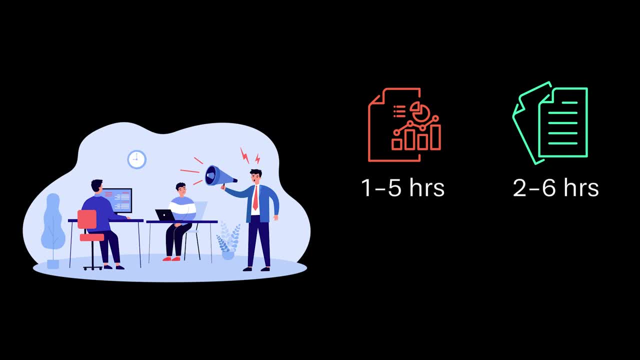 anywhere between one to five and two to six hours respectively to complete, and your performance on one report has no bearing on the other. So those assumptions are going to inform the first step of Monte Carlo Simulation, which is we will come up with some measure of uncertainty for each. 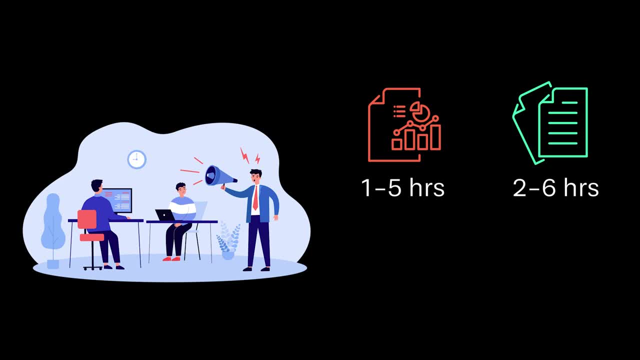 uncertain factor underlying our decision-making process. So, based on a quick search online, you decide to represent the time to complete each report as, following what's called a uniform distribution, which is a really intuitive idea, The probability distribution assumes the relative likelihood of all outcomes between a 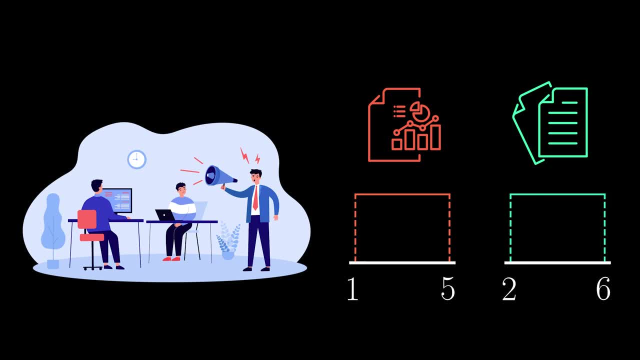 defined min and a defined max are the same. Now, here is where the beauty and simplicity of Monte Carlo Simulation comes into play. What we're going to do now is rely on a computer to randomly pick the time to complete each report. Those selected values are going to be based on. 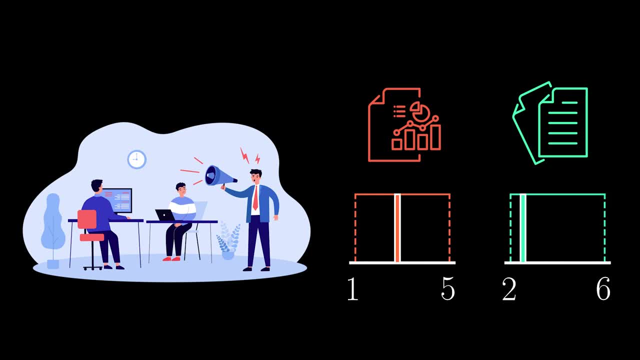 our defined uniform distributions, which is what we're going to do now. So we're going to do a random distribution, which is why it is really important to make sure that you come up with a good estimate of those distributions at the start. Now let's speed this process up and do it. maybe. 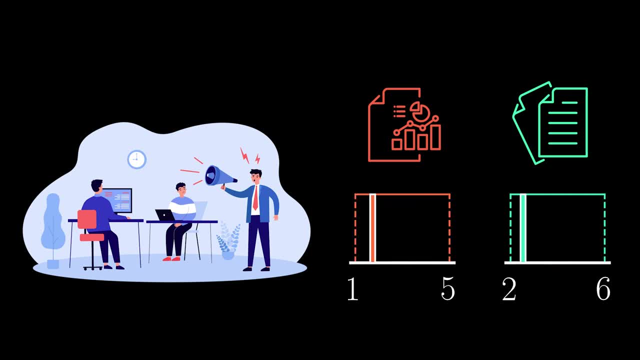 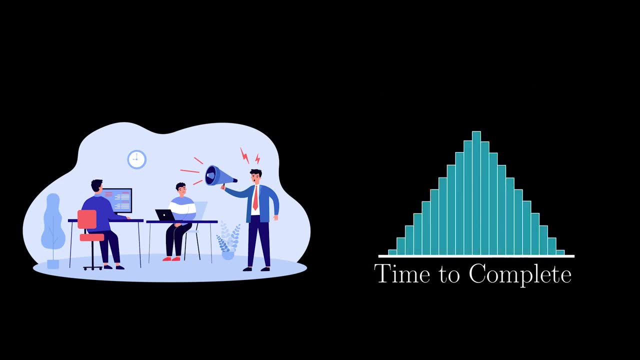 thousands, maybe millions of times, And we're going to store all of these randomly selected values And once we do that, we can use those stored results to approximately estimate the distribution around the time, to complete both reports which we can now use to figure out the 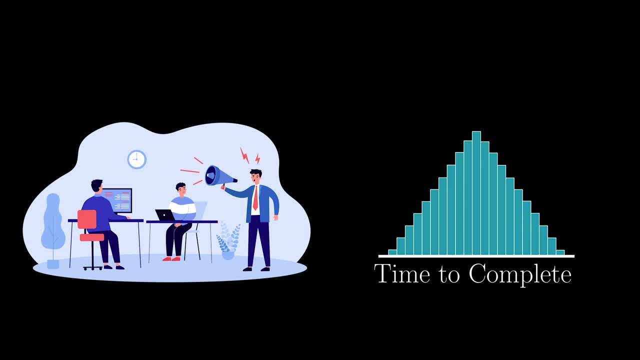 chance we'll make it to the party in time, And that's really the crux of Monte Carlo Simulation, And so you can use that to figure out the chance we'll make it to the party in time, And that's really the crux of Monte Carlo Simulation, And so you can. 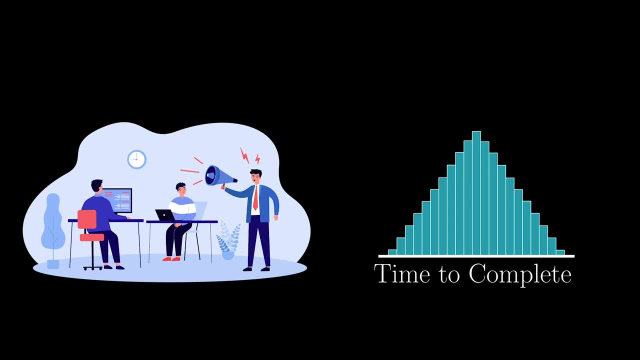 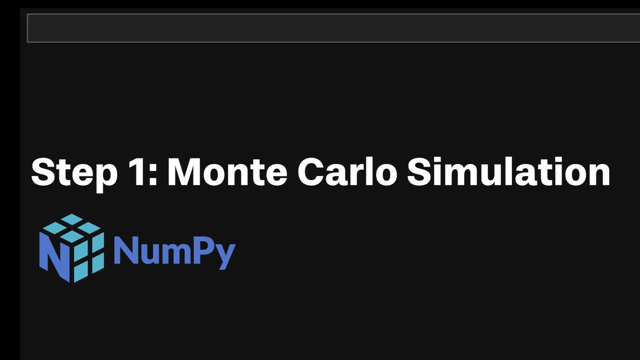 imagine, for problems with many sources of uncertainty. Monte Carlo Simulation provides a simple way to analyze complex systems. So to really appreciate Monte Carlo Simulation, let's quickly show how you can implement it, And I'm going to do so in this video through Python To. 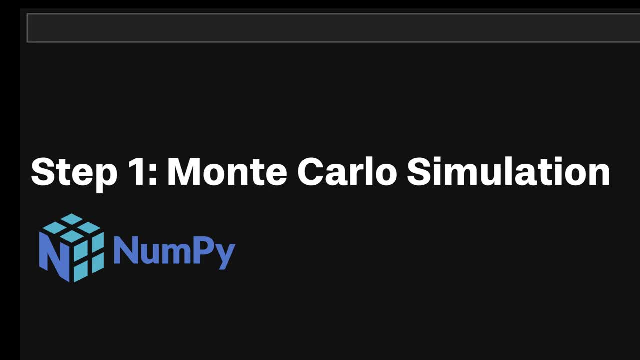 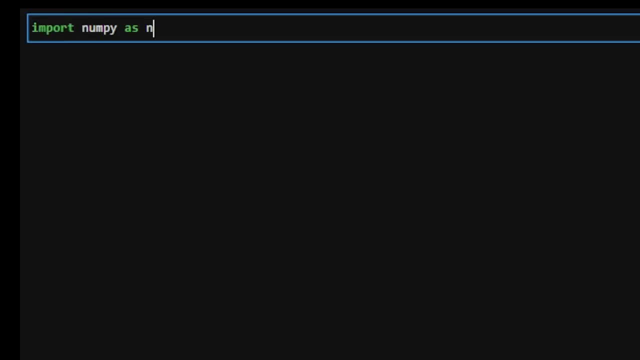 first go about conducting our Monte Carlo Simulation. we're going to rely on a library called NumPy which has available functionality to conduct Monte Carlo Simulation. So I'm going to import NumPy and propose that we're going to use the function numpy to conduct Monte Carlo Simulation. 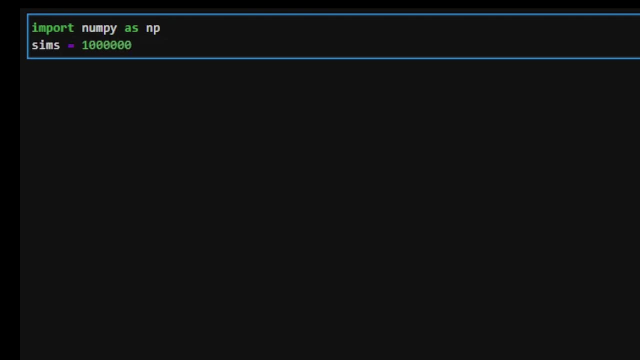 And I'm going to import NumPy and propose that we do 1000.. Let's just make it 1 million. Monte Carlo simulations, And we'll do this for our two reports, which I'll refer to as being A and B, And they will take anywhere between one to five hours and two to six hours to complete. 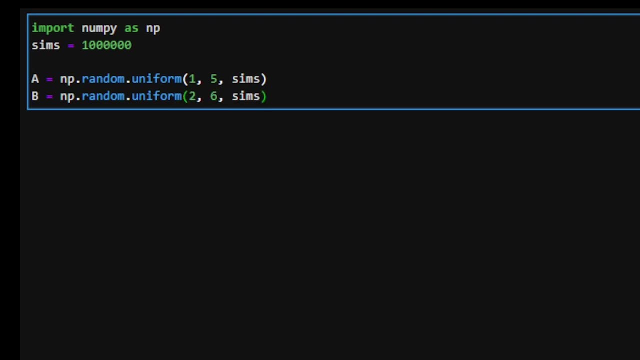 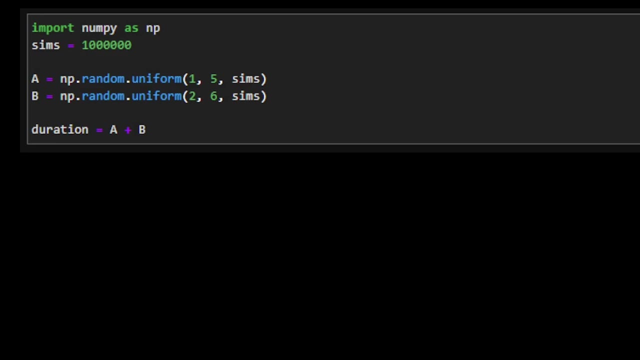 So let's define those values for the arguments for these functions And, of course, the total time to complete these two reports is simply their summation, So let's add them up And voila, we now have 1 million random samples, which is great. 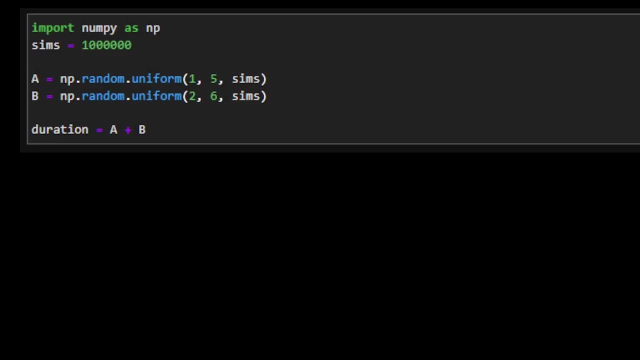 but we now need to be able to use them to properly figure out the chance we'll make it to the party on time. So to do this, what I'll do now is bring in matplotlib, which I frequently rely on to visualize data, And what we're going to do once we've imported matplotlib is initialize a plot. 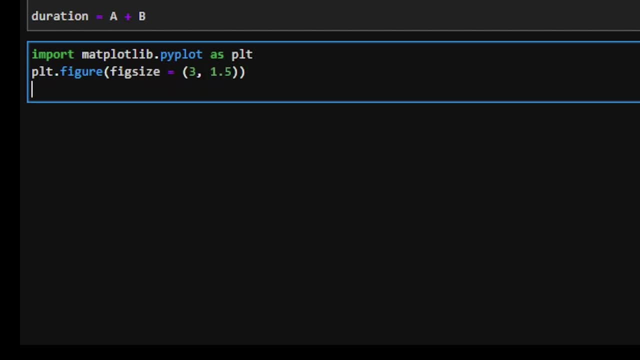 which will be a histogram, And you'll notice that I set the argument density being equal to true, so that we can plot everything in the form of probability densities. And let's also layer on top of this plot a vertical red line at the value nine, as the barbecue is in just nine hours, making it a bit easier to visualize. 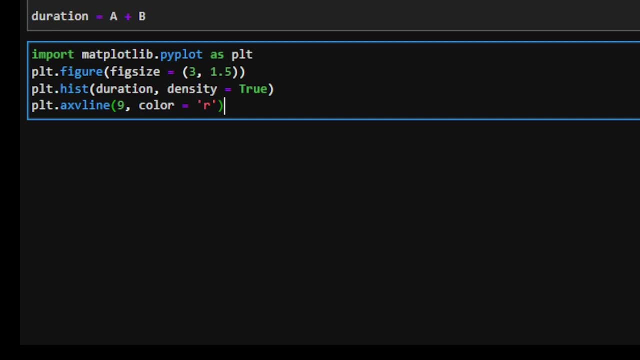 the probability the total time to complete both reports exceeds that threshold. And let's just do one more thing. After showing our plot, let's print the percentage of simulations that exceeded a total of nine hours. We can do this by simply summing up the number of instances that meet a condition. 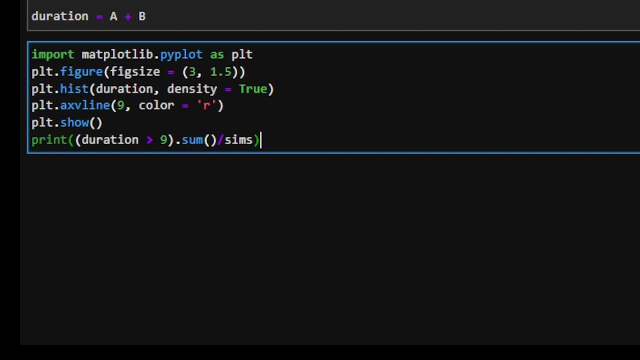 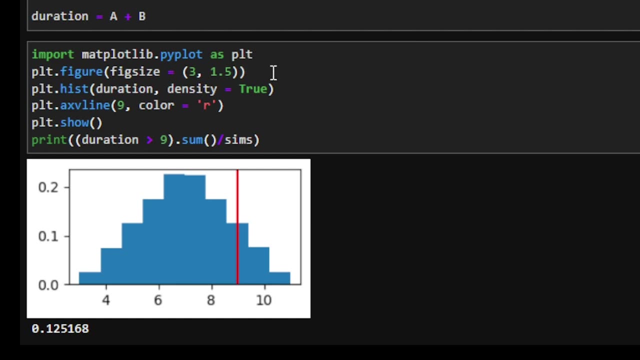 In this case, the time to complete exceeds nine hours, and dividing it by the total number of simulations- And how cool is that? Without doing any hand calculations or derivations, you could pretty quickly estimate that there is a reasonable chance that you won't make it to the barbecue in nine hours. 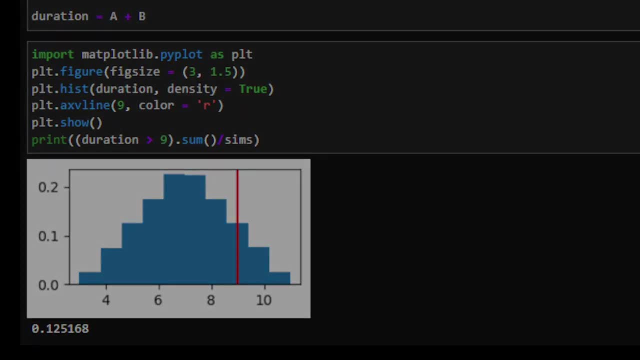 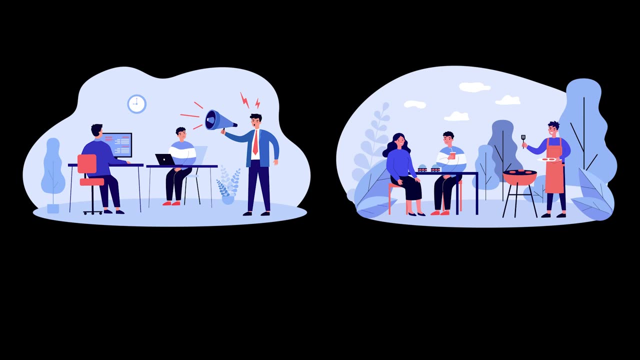 around 12 to 13%. So, based on this probability, should you tell Todd to get lost? Should you take on these two reports, risking the chance that you'll miss out on the party? I'll leave that up to you, But what I can tell you is that Monte Carlo simulation. 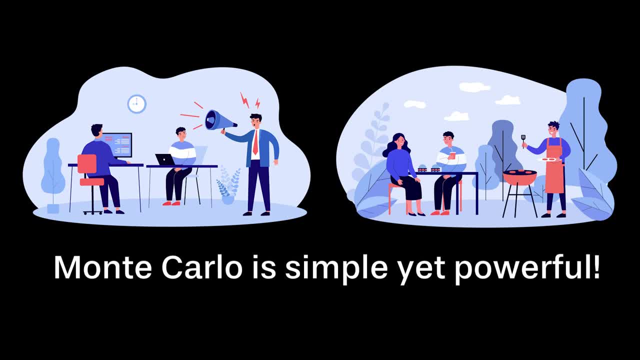 is straightforward and intuitive and can be used to answer probability questions pretty simply, with little required background knowledge of probability, And you can use this information to ultimately make the best choice for you. Now, if you've made it to the end of this video, definitely don't hesitate to subscribe. 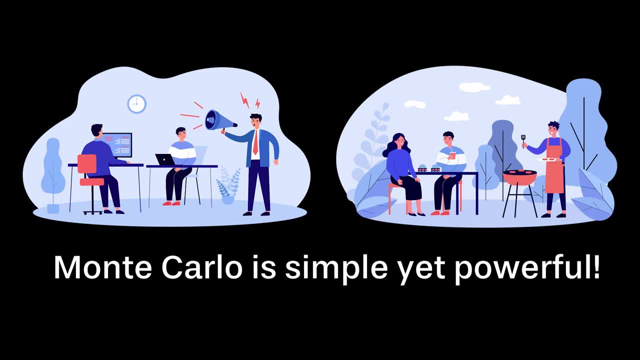 to the channel if you're interested in learning more about this type of content. It definitely helps the channel reach and support a much broader community And, for those interested, I've included a link in the description to the code used in this video. Thank you, as always. 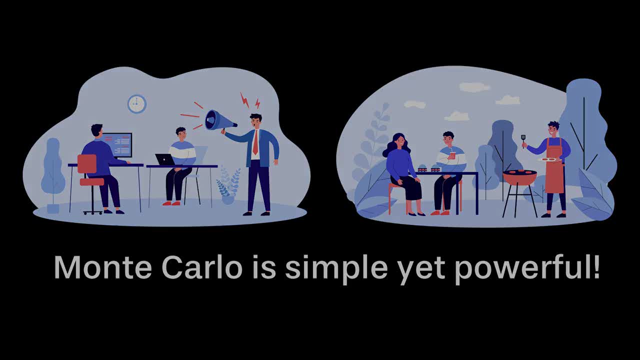 For your interest and support. I look forward to seeing you soon. 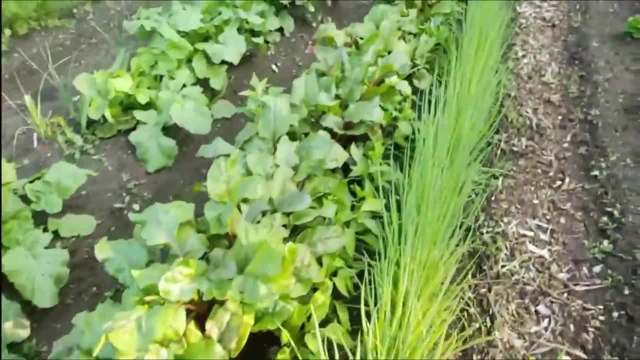 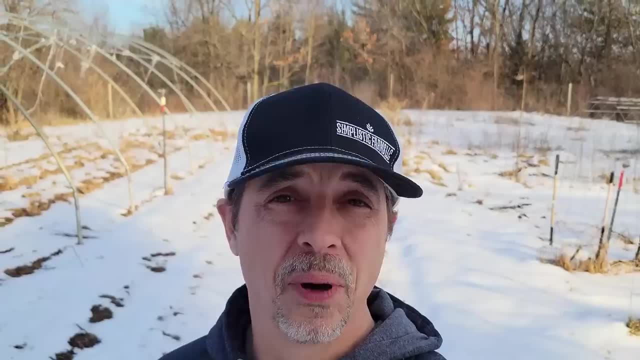 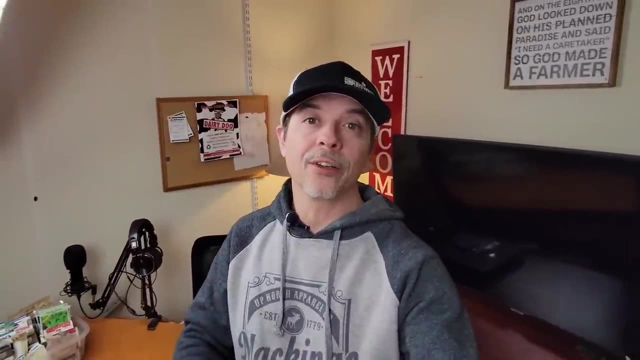 You want to take your garden to the next level. Companion planting might just be the answer, But it's the middle of February in Michigan, so let's take this inside, Alright now. by picking plants that work well together, you can drastically improve your. 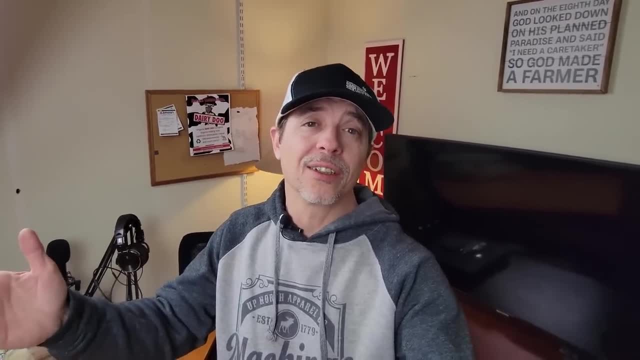 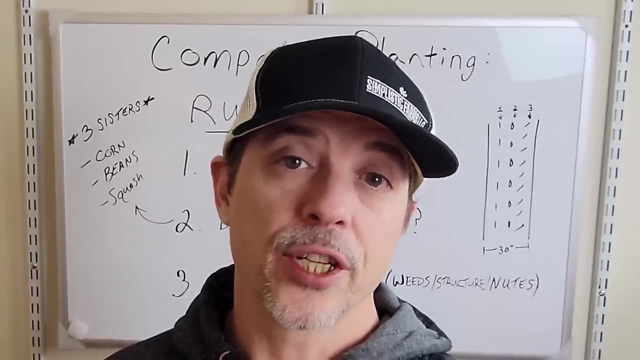 garden's productivity and overall health. But where do you start? Well, that's where the rule of three comes in. By considering just three key factors, you can easily create a winning combination of companion plants. In this video, we're going to show you how to use the rule of. 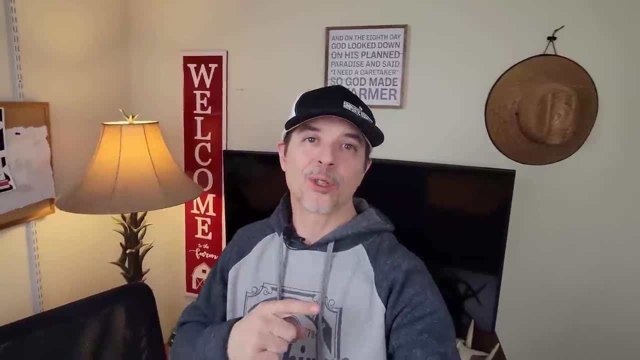 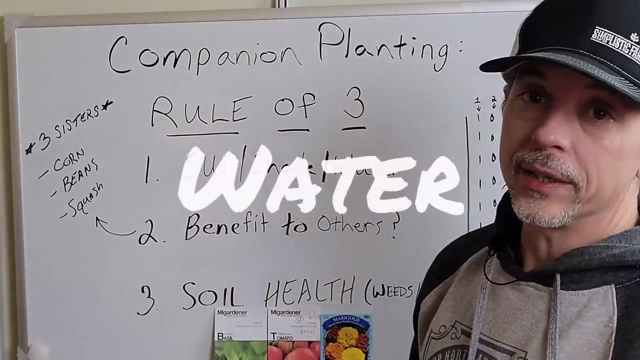 three to make companion planting simple and effective. So let's get started, Alright, now. the first factor that I like to consider is the plant's sun, shade and water needs, And I also look at the plant's height at this time as well. This means that you 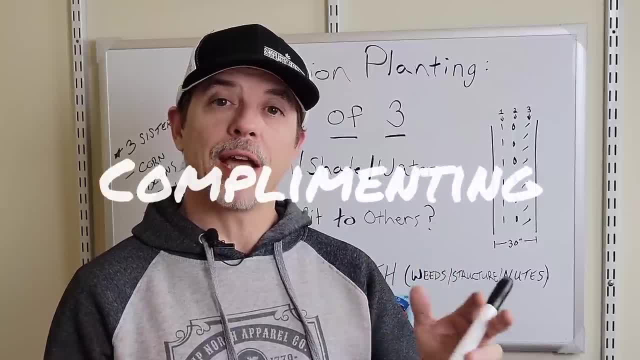 want to choose plants that have similar or complementing shade or sun and water requirements. For example, if you have a plant that needs full sun, you would want to choose a plant that has a similar or complementing shade or sun and water requirements. For example, if you have a plant that needs full sun, you would want to choose a plant that has a similar or complementing shade or sun and water requirements. For example, if you have a plant that needs full sun, you would want to choose a plant that has a similar or complementing shade or sun and water requirements.